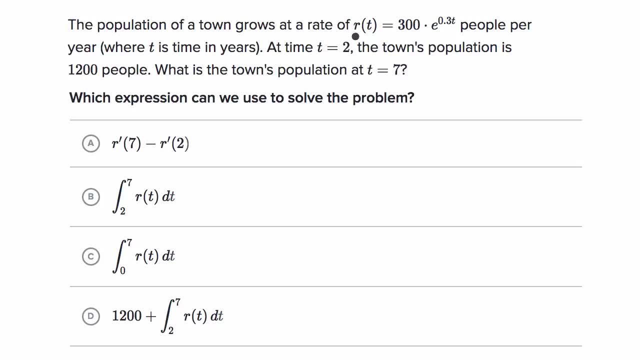 The population of a town grows at a rate of r of t is equal to 300 times e to the 0.3 t people per year. where t is time in years, At time t is equal to two. the town's population is 1,200 people. 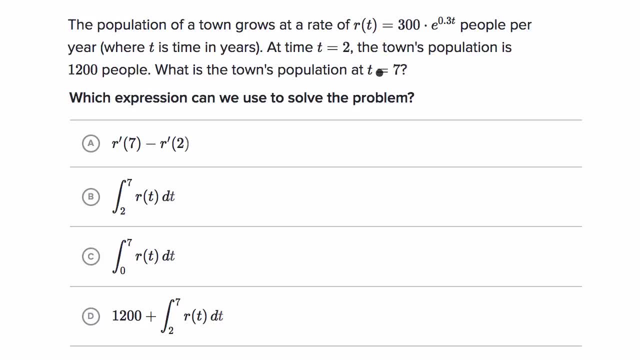 What is the town's population at? t is equal to seven. Which expression can we use to solve the problem? So they don't want us to actually answer the question, They just want us to set up the expression using some symbols from calculus. So why don't you pause this video and try to think about it? 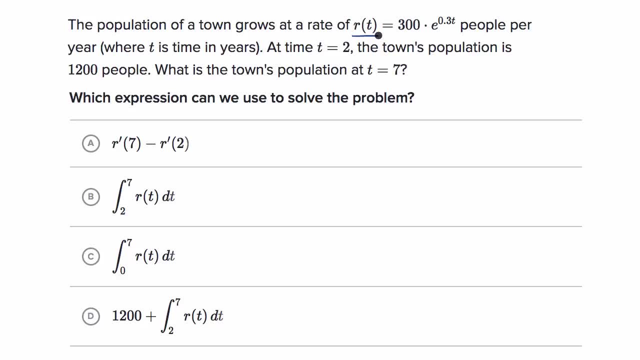 So let's just remind us what they've given us. They've given us the rate function right over here, And so if you want to find a change in population from one time to another time, what you could do is you could take the integral. 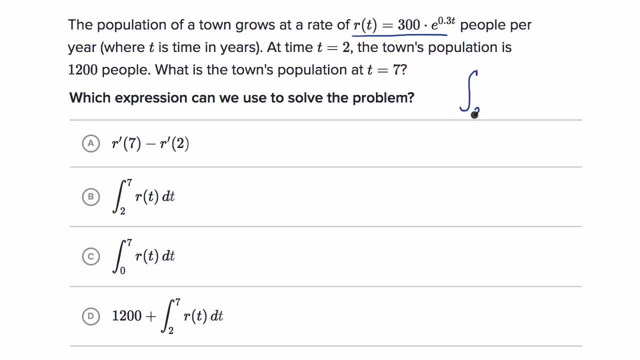 of the rate function from the starting time- t is equal to two years- to t is equal to seven years. So we're gonna take the integral of the rate function and what this is going to tell us. this is going to tell us the change in population. 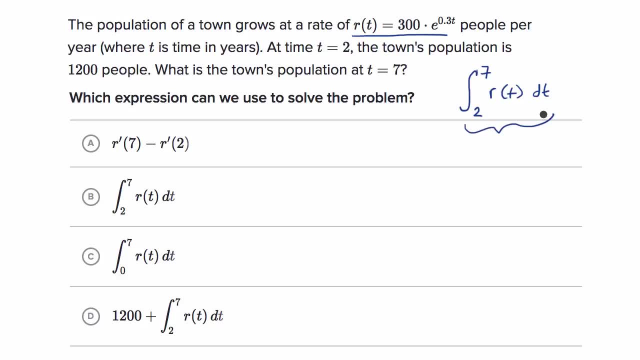 from time two to time seven. So this is. you could say, let me just write this, This is the change. I'll use delta for change, or I'll just let me just write it out. Change in population. change in population. 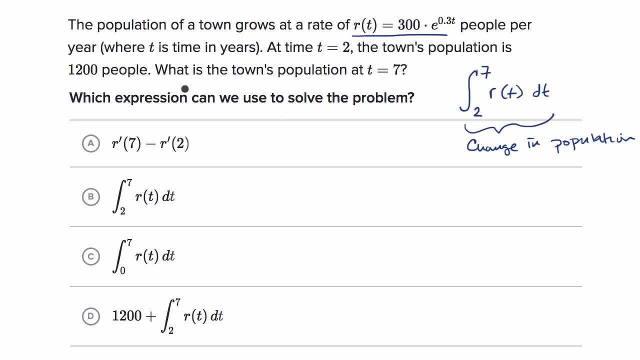 Population, But they don't want us to. they're not asking us for the change in population. They want us to know what is the town's population at t is equal to seven. So what you would want is you would want what your population is at. t equals two. 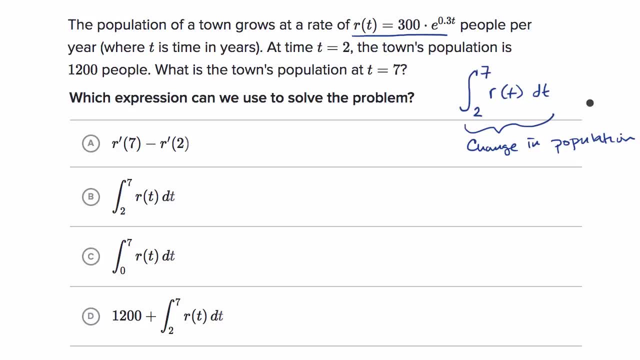 plus the change in population from two to seven to get you your population at seven. So they tell us the population at time. t equals two. the town's population is 1200 people. So if you want, the population at t is equal to seven. 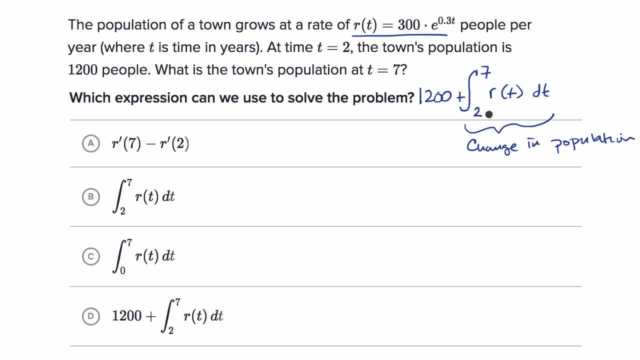 it's going to be 1200 plus how, whatever the change in population, if you take the integral of the rate function you are, and this is the rate of population- this integral is going to give you the change in population from time t equals two to t equals seven. 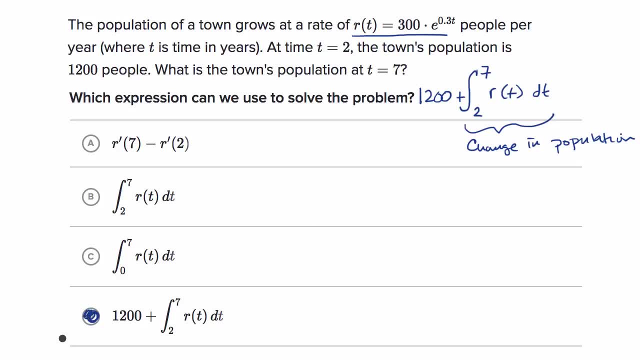 So we can see clearly that is choice D right over here. These other choices, we can look at them really quick. Choice B is just the change in population That, assuming that this is and this is actually increasing. so this would tell us how much did the population increase? 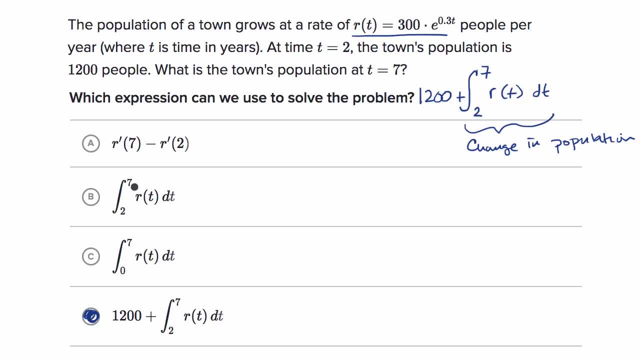 from from t equals two to t equals seven. So that's not what we want. We want what the actual population is. This is how much the population increases from time zero to time seven. Now you might say, well, wouldn't that be the town's population? 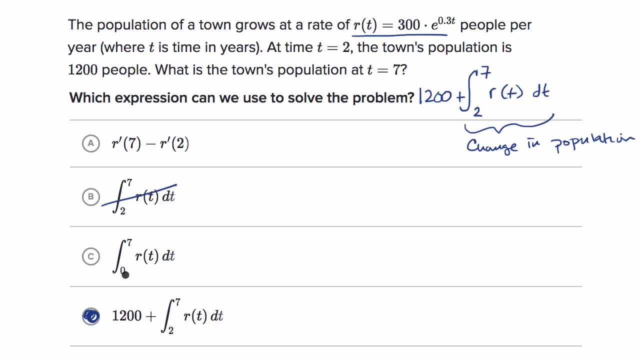 Well, that would be the town's population if they had no people at time zero. but you can't assume that Maybe the town got settled by 10 people or by a thousand people or who knows whatever else. So right over there- And this is taking the derivative of the rate function, 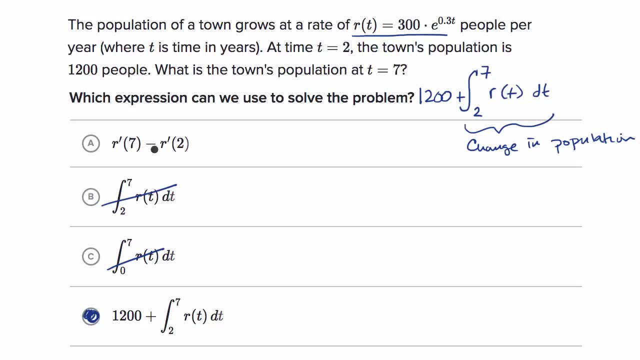 which is. it's actually a little hard to think about. what is this? This is the rate of change of the rate at time seven minus the rate of change of the rate at time two, So I would rule that one out as well. Let's do one more of these. 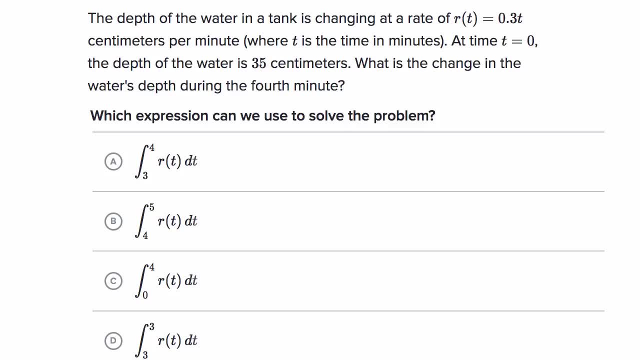 So here we have. the depth of water in a tank is changing at a rate of r of t is equal to 0.3 t centimeters per minute, where t is the time in minutes. At time, t equals zero. the depth of the water is 35 centimeters. 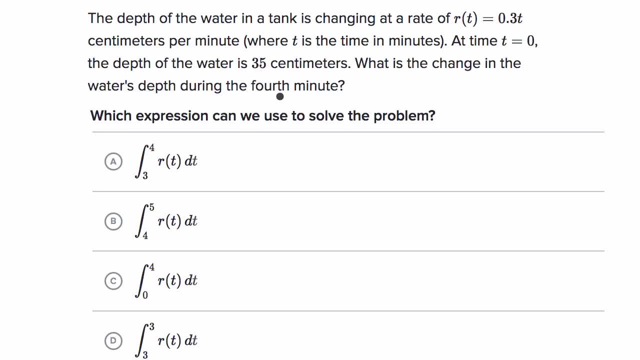 What is the change in the water's depth during the fourth minute? So let's pause the video again and see if you can figure this out again, or figure out what expression can we use to solve the problem, The problem being: what is the change in the water's depth? 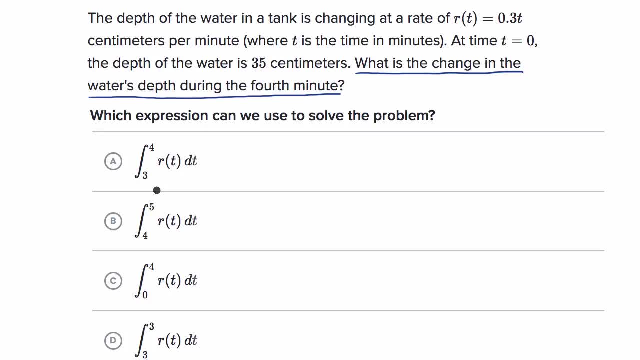 during the fourth minute. All right, So we've just talked about. if you're trying to find the change in a value, you could take the integral of the rate function over the appropriate time. So we're talking about during the fourth minute. 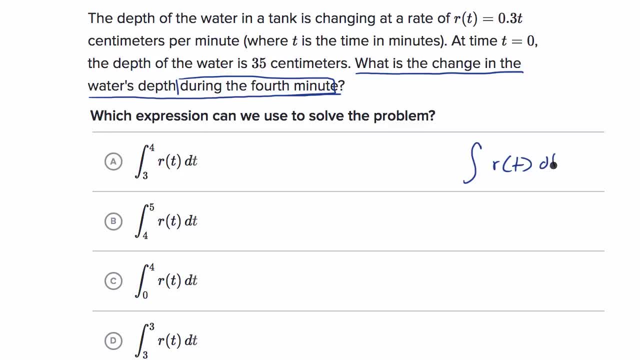 So we definitely wanna take the integral of the rate function And we just have to think about the bounds and all of the choices here are taking the integral of the rate function. So really, the interesting part is during the fourth minute, So let me just draw a little number line here. 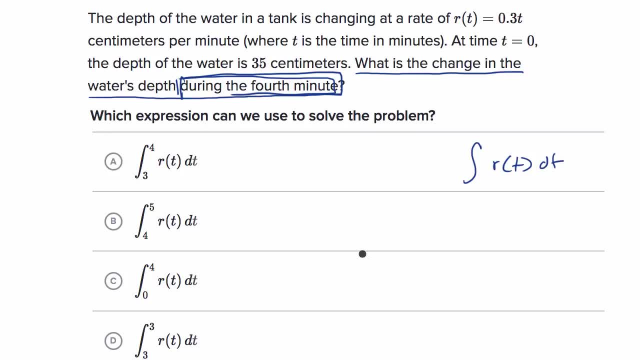 We could think about what the fourth minute looks like, Or actually let me just draw the whole thing. So let's say: this is r of t, right over there. Or you could say y is equal to r of t And this is t. 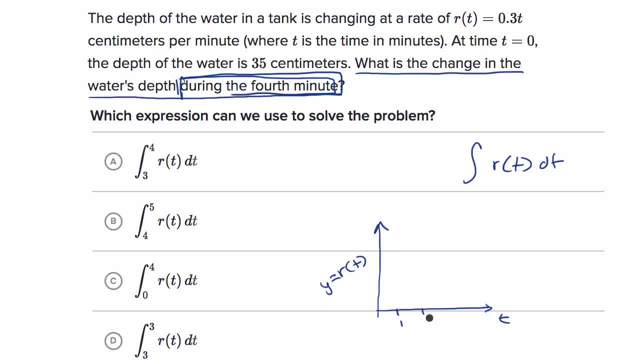 And let's see: The first minute goes from zero to one. Second minute goes from one to two. Third minute goes from two to three. Fourth minute goes from three to four. The rate function. this actually just looks like a straight up linear rate function. 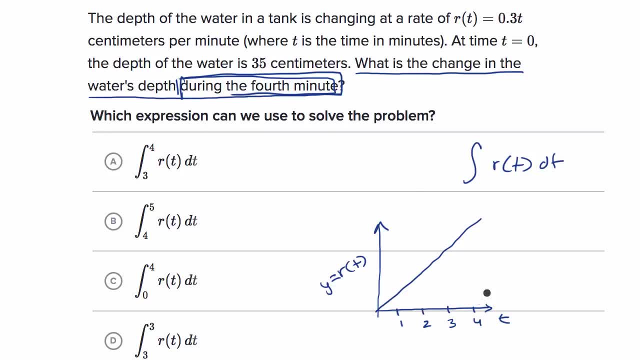 looks something like this. And so what is the fourth minute? Well, the fourth minute is the first minute. is this one? Second, third, fourth. The fourth minute is going from minute three to minute four. So it's what we wanna do, is the expression that gives us. 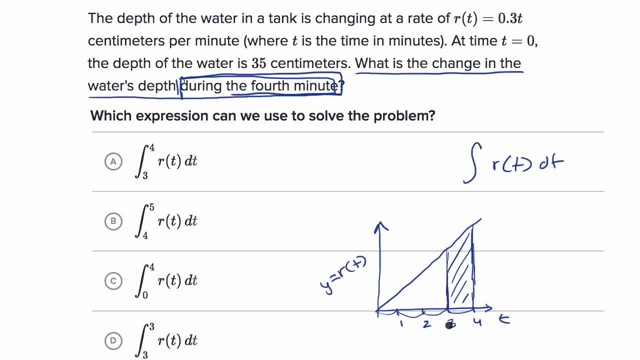 this area right over here under the rate curve. Well, this is, our lower bound's going to be three, and our upper bound is going to be four, And so there you have it. It is this first choice. You might have been tempted here. 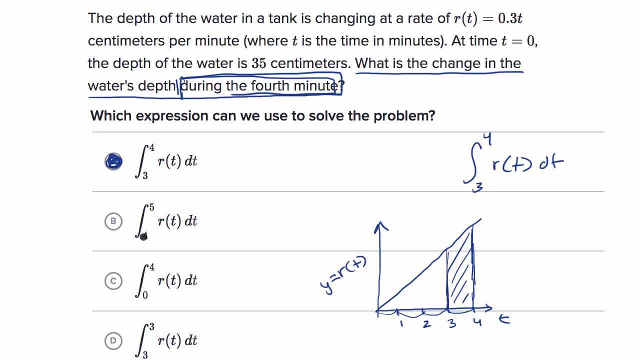 if you got a little bit confused. Hey, maybe the fourth minute is after we've crossed that. t is equal to four, But no, that would be the fifth minute. This would tell us our change over the first four minutes, not just during the fourth minute. 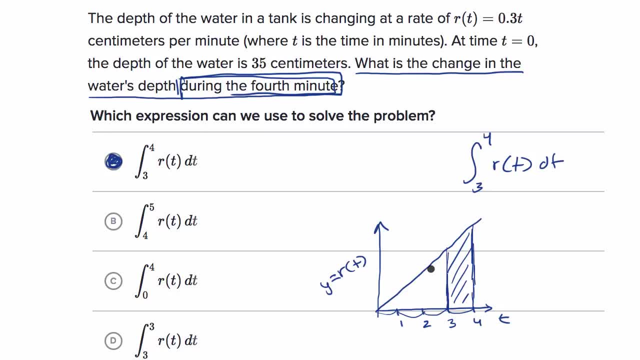 And then this: well, this is just gonna be zero. If you're taking, this is what is the change in the value from three to three? Well, it didn't change at all in that, because it's essentially at an instant.